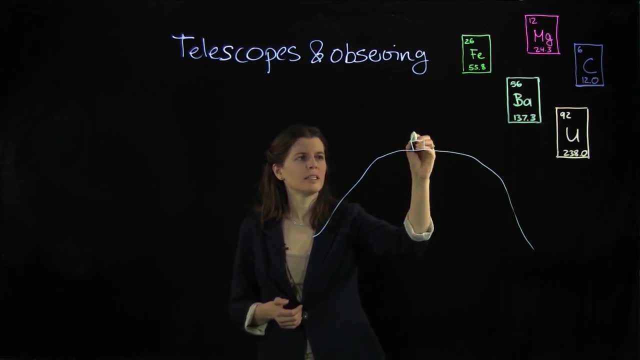 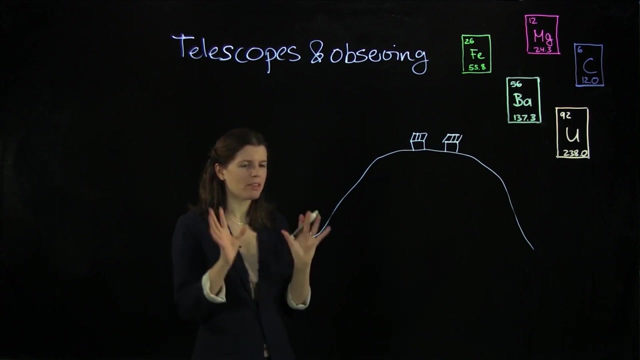 and you see a little telescope glistening in the sun. Actually, there are two telescopes there, the twin telescopes. I use mostly just one of them. sometimes I use the other one too, and one time actually I used them both. that was exciting, both at the same time. 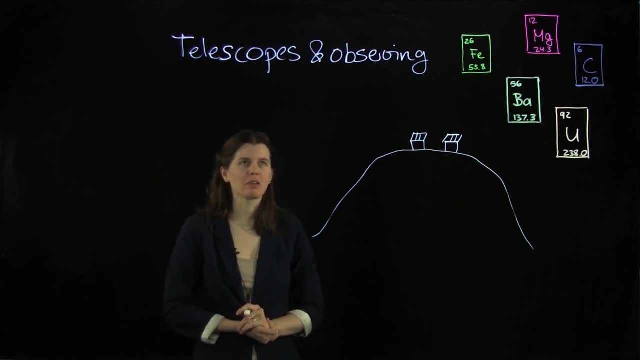 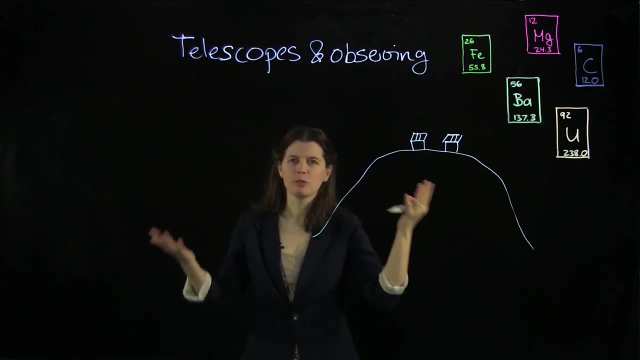 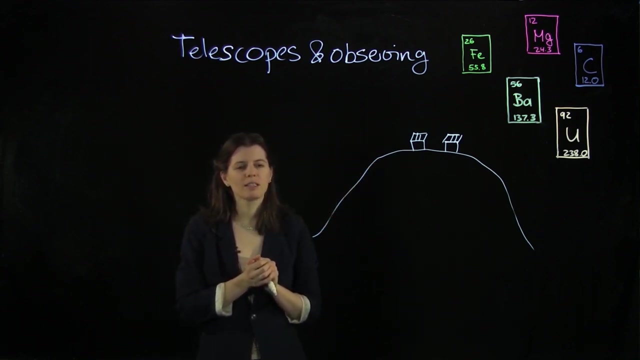 I had to run back and forth between the two to make sure that everything is working properly and what? what you have when you get there is that you have a beautiful mountain landscape and, of course, at night, you have the beautiful dark sky above you and the stars are so bright. 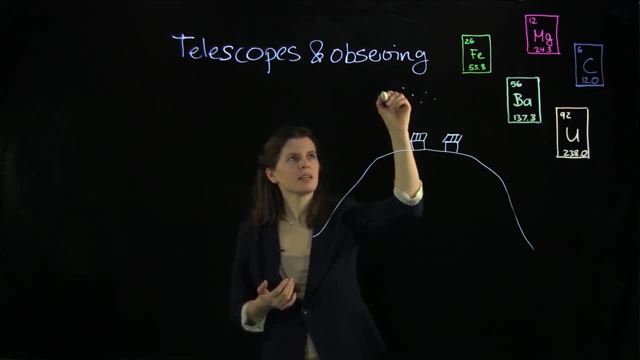 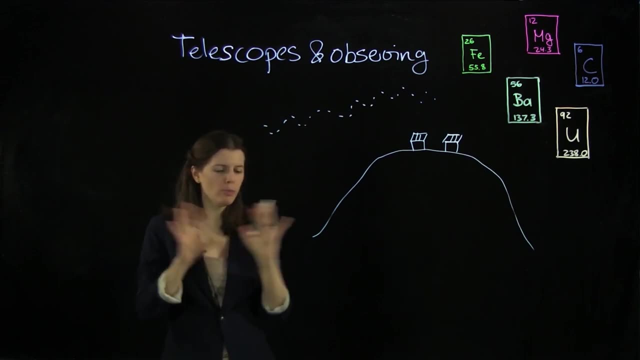 all together when they make up the milky way that actually, I used to walk outside and I didn't need to bring a flashlight. I didn't need to bring a flashlight. I didn't need to bring a flashlight. There was no moon, but the milky way band in the southern hemisphere is so bright. 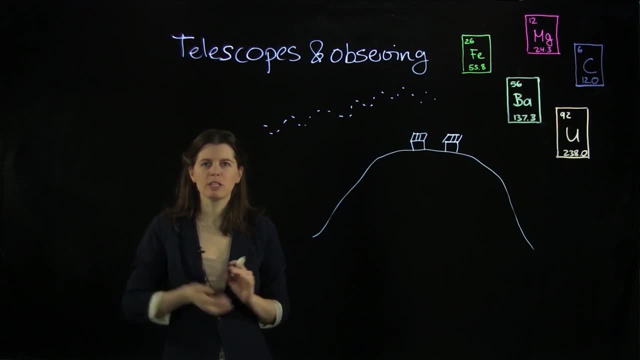 that you can just walk outside. you wouldn't run into a tree or a car or whatever, and I could almost imagine that I would see the shadow from the milky way's light. I could have just imagined that, but the fact that I actually was in this position. 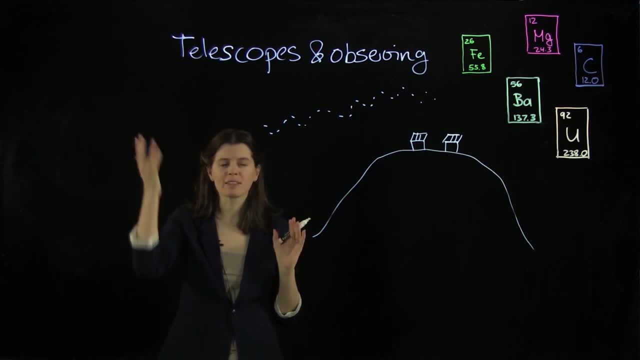 that I said like, oh, can I see my shadow from the, from the night sky? that's just fantastic in itself. So in the following I want to show you a few videos that I have taken at the telescopes to give you a little insight into what it means.